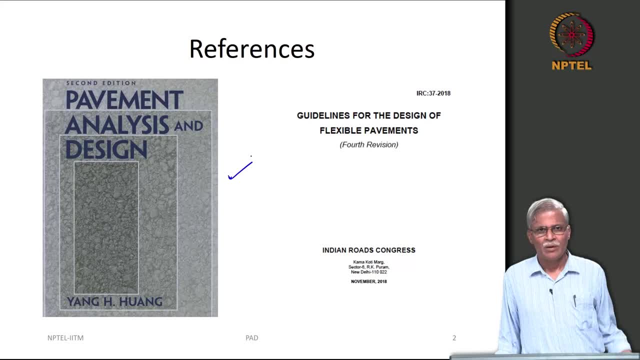 And here also, Professor Huang passed away an year back, So, but as of now, this is the current and latest reference for this. In addition to this, what you really need to do is to get IRC37-2008.. This is the latest guideline for the design of pavements. 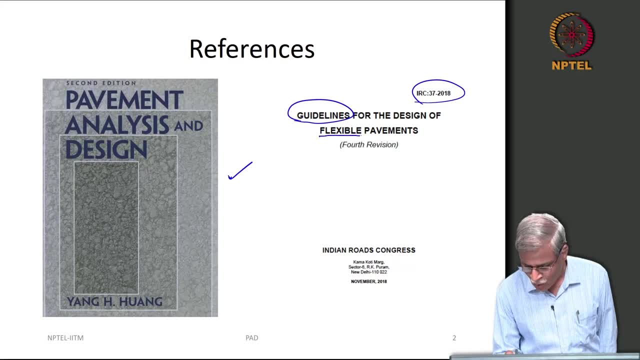 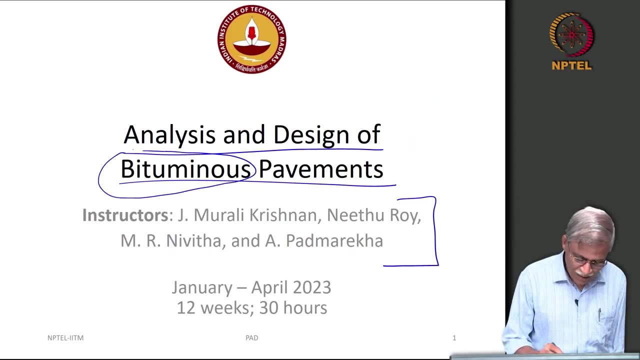 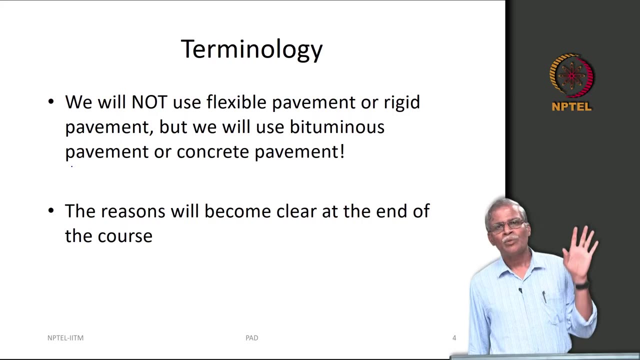 So now You will be be in curious to know that they have written it here as flexible pavement and I have written it here as bituminous pavement. Throughout this course we will be using only this terminology. we will use only bituminous. 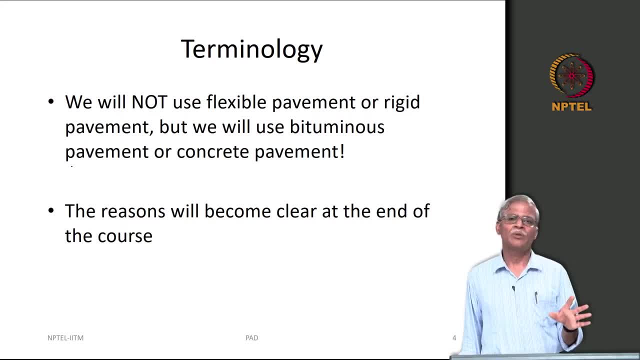 pavement and concrete pavement, and not flexible pavement or rigid pavement. Of course, this course is only about bituminous pavement. sometimes later, we will also be offering something on concrete pavement in a much more rigorous way, But as of now we will be talking about bituminous pavement and the terminology that will be. 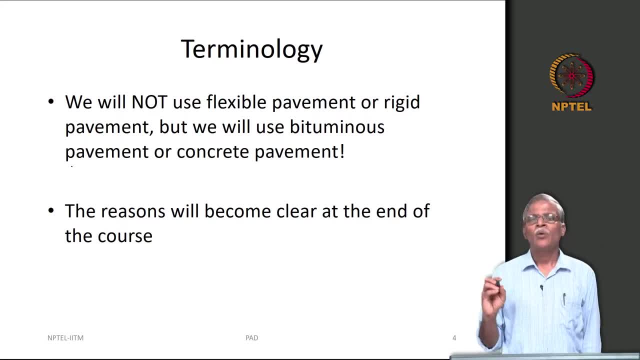 used is only bituminous pavement. Now the reasons will become obvious to you as we go along, but I just want to give a hint. The reason why one should stick to bituminous pavement or concrete pavement is basically related to the stress analysis procedure that is followed. 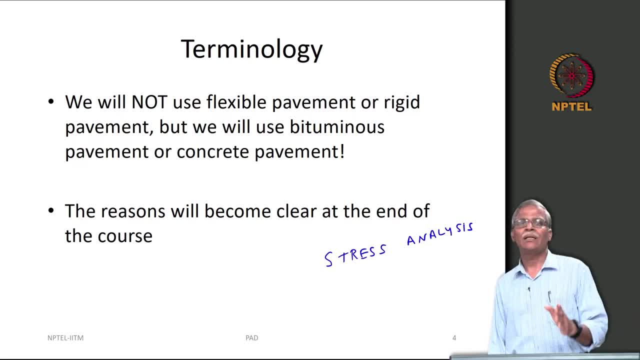 For bituminous pavement, we use what is really called as layered linear elastic theories. For concrete pavement, we use what is called beam on elastic foundation- Winkler model, Pasternak model and all those things. So now it is possible that you can model concrete pavement using layered elastic theories. 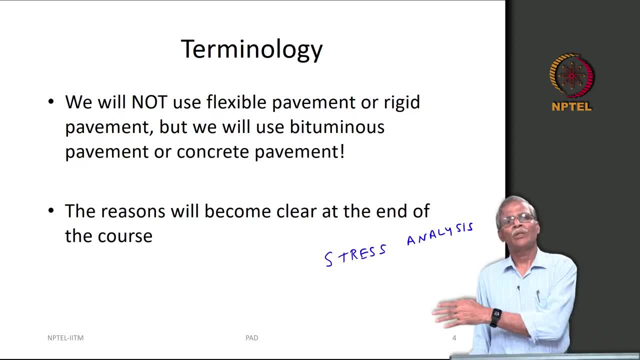 It is also possible that you can model bituminous pavement using the Winkler model. Thank you, So there is nothing flexible or nothing rigid about it. Now, what are all the things that we are going to do here is? we will first look into the 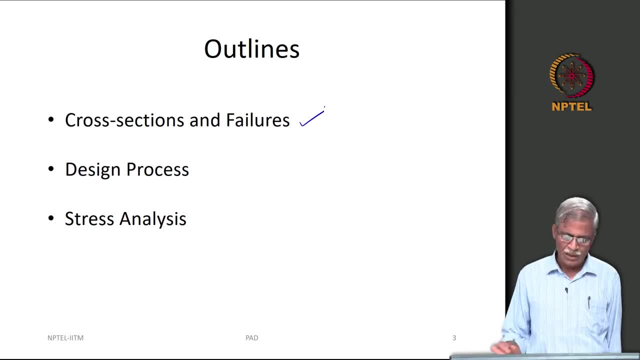 various cross sections and how a pavement fails, Then we will be talking about the overview of the design process and then we will talk about the stress analysis. Now you must be actually wondering as to why I first talk about failure And then talk about the design process. and in fact, many a time you will notice that, and 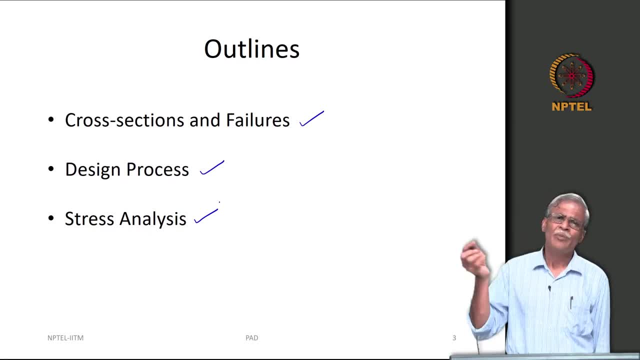 this holds good not only for pavement engineering, but also for many civil engineering infrastructure. What we do is always what is really called as proof checking, So that means most of the time, based on the past experience, we have a very clear cut idea of What should be the kind of layer thickness that should be provided. 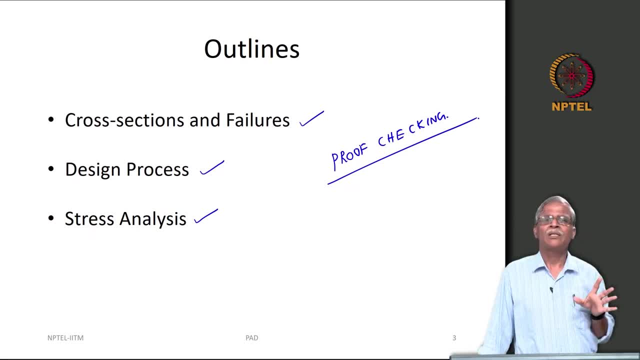 So most of the time this comes more from the constructability aspect. Obviously, when you are constructing a pavement, you are not going to tell your highway engineer to construct 45.22 mm layer thickness. That is not going to be possible. The nominal maximum aggregate size, the ability of the roller to compact, the relation between 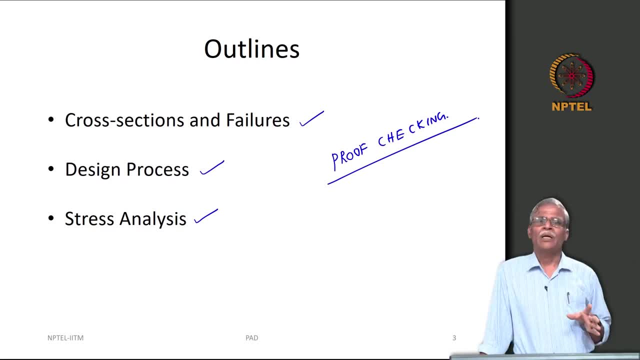 the maximum aggregate size to the layer thickness. All of these things play a critical role. So what we first want to find out is: these are the different cross sections, and each cross section has a specific. each layer in a cross section has a specific role to play. 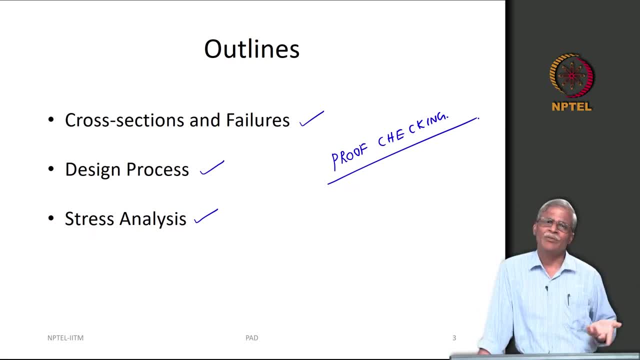 So we will first understand intuitively what really are the failure conditions. Then we will try to compute the critical stresses and strains related to those failure criteria, And for that we need to use a stress analysis procedure. So that is the outline that I am going to take here. 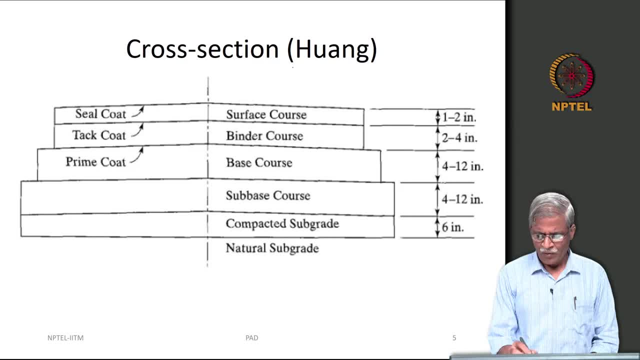 Now very simple cross section, which is listed in Hoang, and more or less this is the standard cross section that is followed. You should be little bit careful about the units that are used here. This is an American textbook, So most of these things are given in terms of inches, even in some of the example problems. 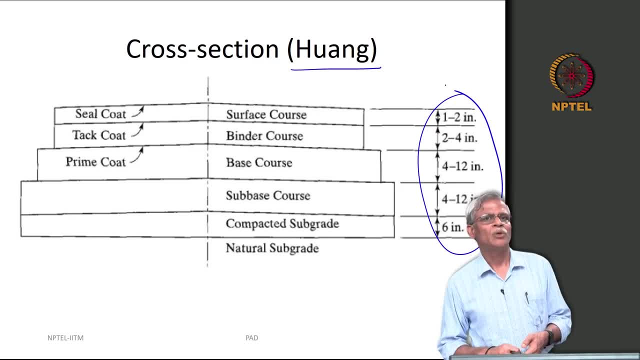 that you will be working out from this textbook, Okay, Which will be shared with you. The units will be mostly pounds inches, But we will also be providing the conversion within the bracket, So do not worry about it. So if you go from the bottom, you are talking about a natural sub-grid. 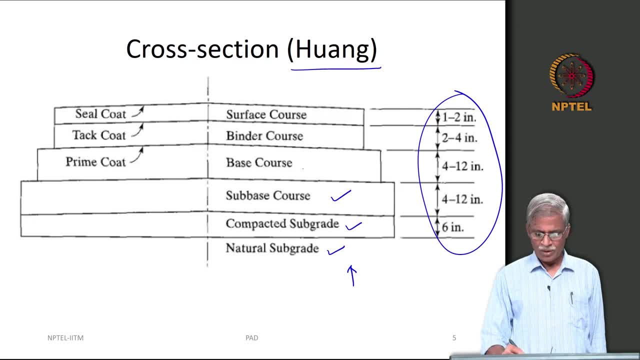 Then you talk about a compacted sub-grid: a sub-base, a base, a binder and a surface. Now these two layers are connected. These two layers are bituminous in nature predominantly, Then these three layers are granular material and then you also have a prime coat between. 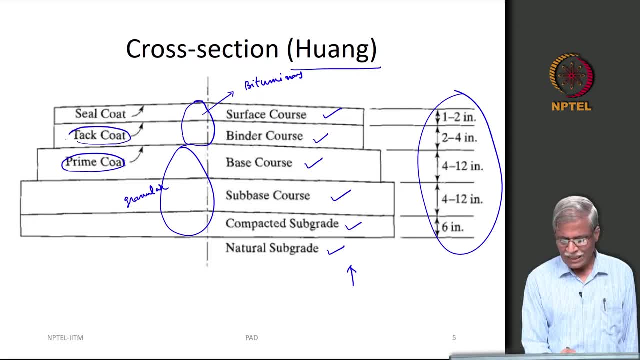 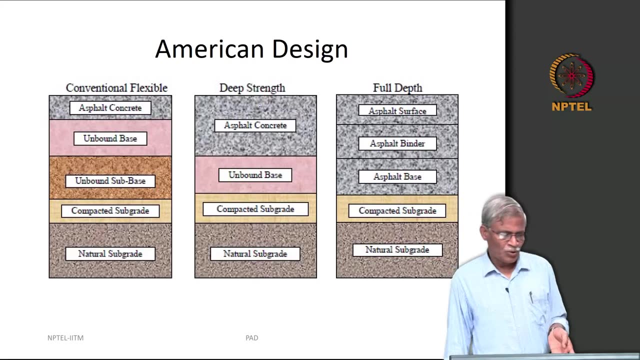 the base cores and the binder cores, a tack coat between the binder cores and the surface cores, Okay, Okay, So you can provide a seal coat, but you can actually see that it is provided here Right Now. this is the general cross-section that you saw. 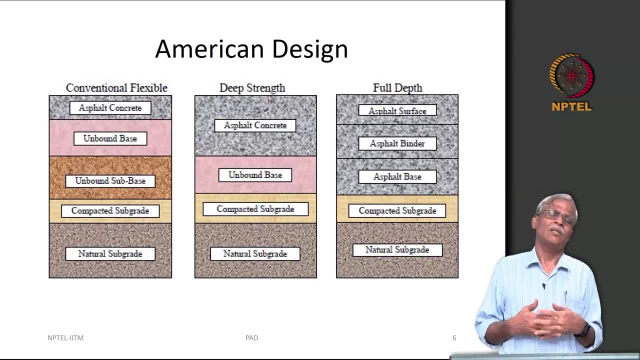 But if you take a look at the typical cross-section that is provided in American roads, which is most of the design procedures that follow AASHTO and what we call as MEPDG- Mechanistic Empirical Pavement Design Guide, So you will see that 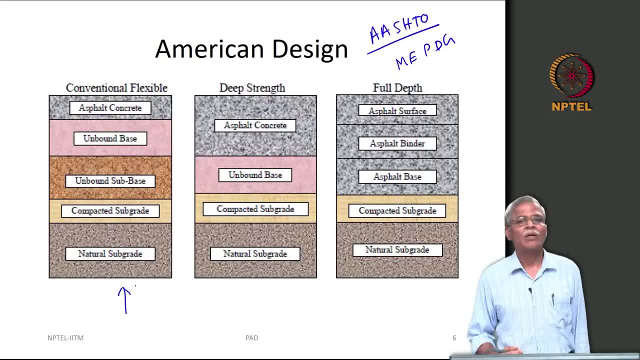 There is a conventional flexible pavement. Now this is we call it as asphalt pavement or bituminous pavement. Okay, So what you are going to see is there is a natural sub-grid, There is a compacted sub-grid, unbound sub-base. unbound base: unbituminous mixtures or asphalt. 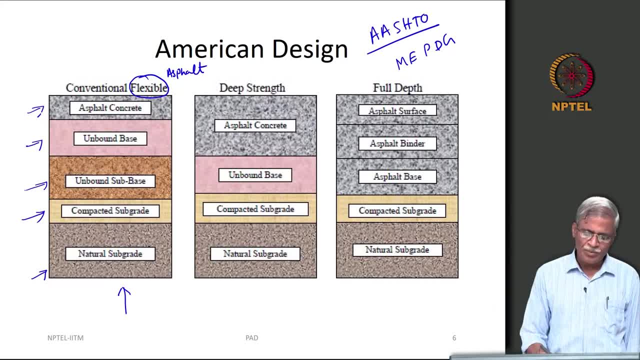 concrete mixtures. Okay. So this is something similar to the generic cross-section that was presented to you earlier. Now there is something called as a deep strength pavement- Okay, Perpetual pavement, and all those things. So you will see that it is the same. the natural sub-grid. The compacted sub-grid has a slightly more thickness. This is the unbound base, And then what you are going to see here is: Okay, The thickness of the asphalt concrete layers are substantial. More or less. it consists of the layer thickness of the unbound base as well as the asphalt. 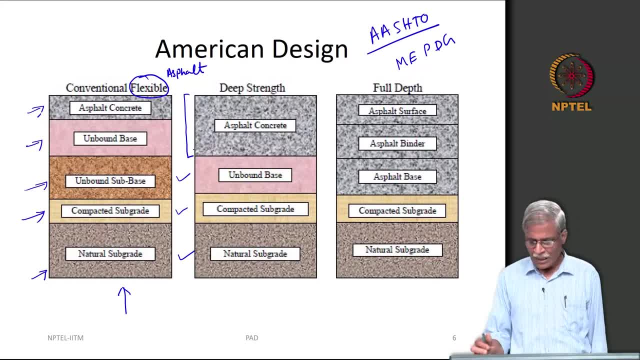 concrete. Okay, So this is the deep strength pavement. In addition, of course, you have what is really called as a full depth pavement, and such kind of pavement were propagated by asphalt institutes- Asphalt Institute of United States. So this is a non-profit organization which is basically promoting the asphalt related 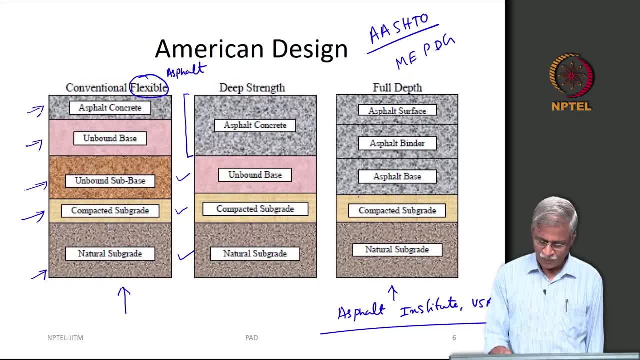 products. So you will see that everything is asphalt. So what you really see is a compacted sub-grid. Then you have an asphalt base, asphalt binder course, asphalt surface course. So obviously the cost of these constructions are going to be very, very expensive. 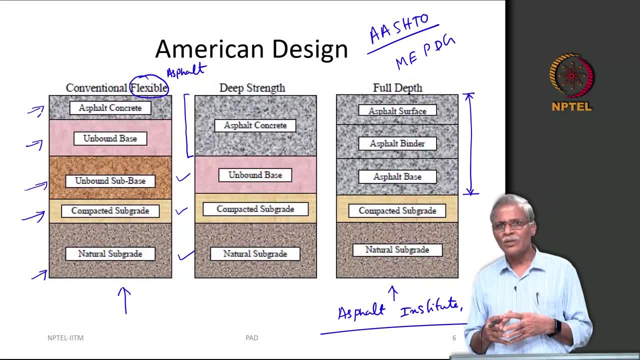 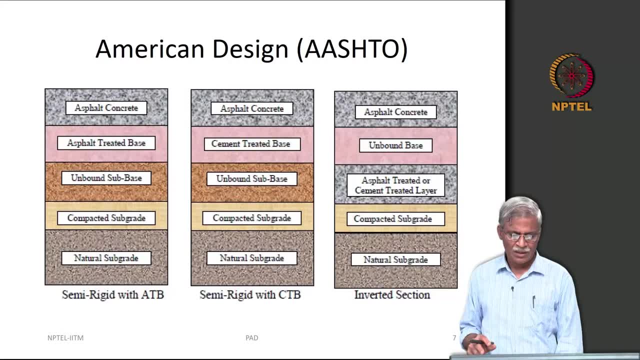 Some of these constructions are normally used in runways, sometimes in heavy duty industrial flooring. Okay, So that is the American design. Then you also have different inverted cross sections here, So we will go from this side. Okay, So there is an actual sub-grid. 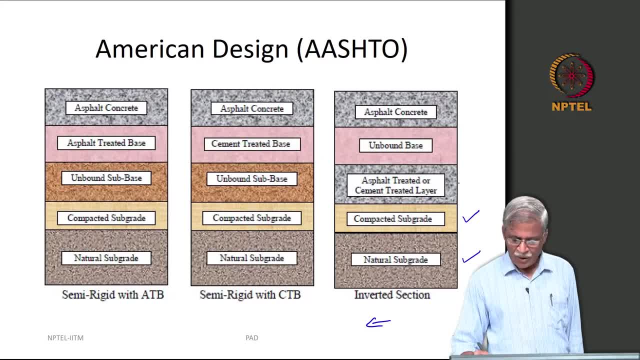 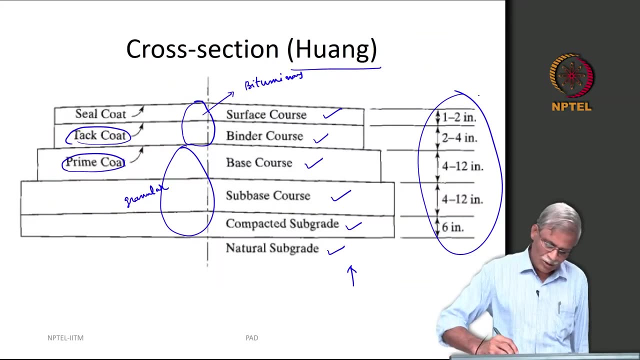 There is a compacted sub-grid. Then you have a cement treated layer and an unbound base and an asphalt concrete layer. Okay, Now why is this called as an inverted layer? Now, the common tendency here is to see that, as you go from the bottom to the top, the 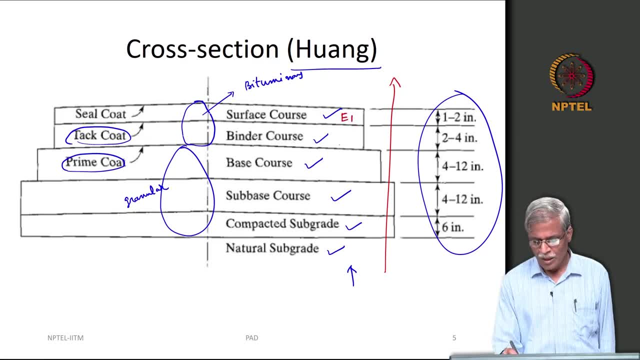 modulus value keeps increasing. So if you call this as E1, E2, E3, E4, E5, you are going to get see these kind of relations. So the topmost is going to be the material having a higher modulus. 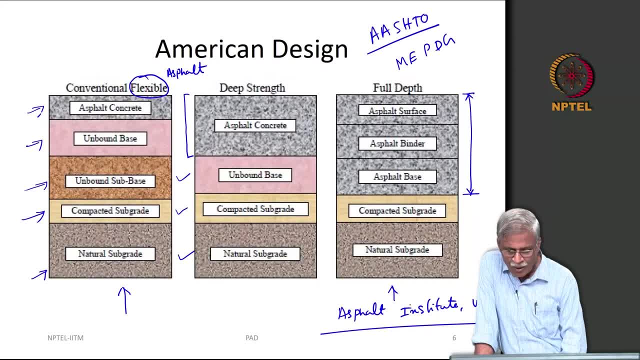 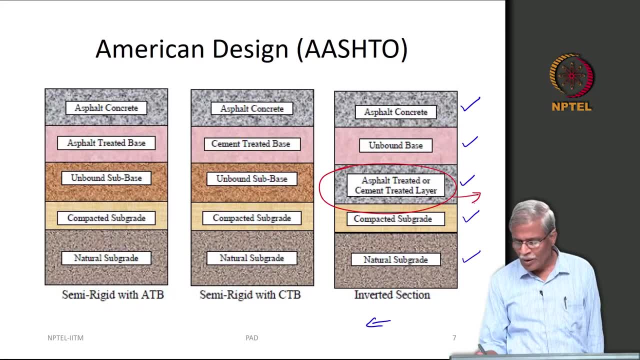 Now, what exactly is the modulus? We will worry about it later, But what you see here is this particular layer. This particular layer can actually have a modulus value slightly higher than this unbound base, And so that is why these sections are actually called as inverted sections. 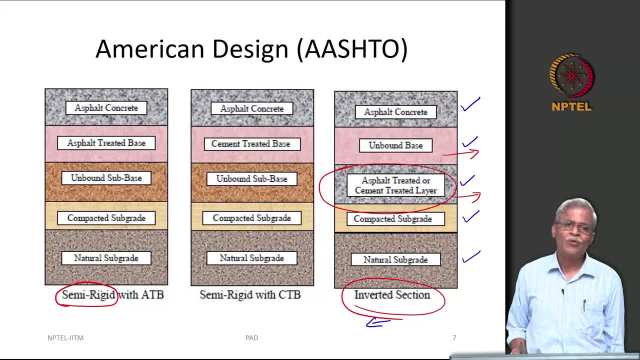 You can… And then- this is an unfortunate terminology- what is called a semi-rigid. or you can say a combination of concrete and bituminous pavement, because bituminous pavement, bituminous pavement- And then you can actually have what is really called as an unbound sub-base, compacted sub-grade. 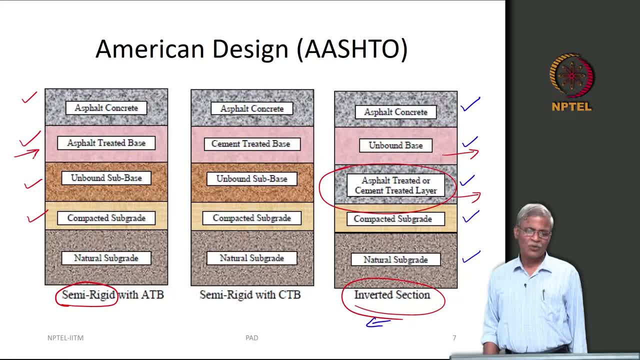 But the most important thing that you see here is an asphalt-treated base. So it is not really a full bituminous mixtures except… But you kind of try to use some amount of bitumen in it. That bitumen could be in the form of a foam. 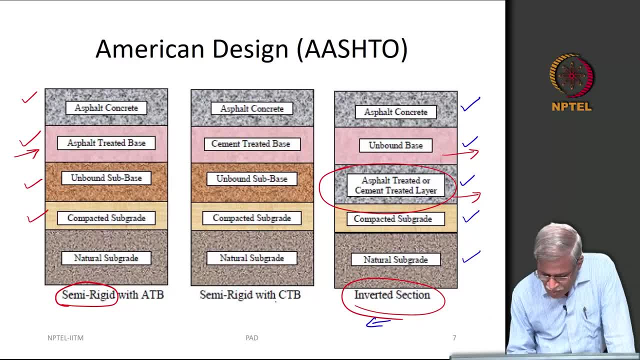 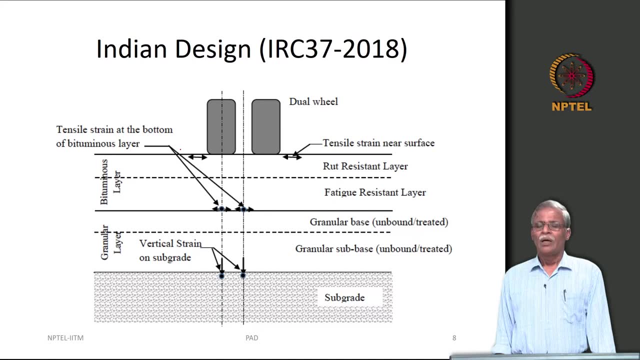 It could be in the form of an emulsion. Now, this is your cement-treated base, Using an asphalt-treated base that you see here. you use a cement-treated base here. Rest of the cross-sections are more or less the same. So let us come to the IRC 37-2008 cross-section and see what it says. 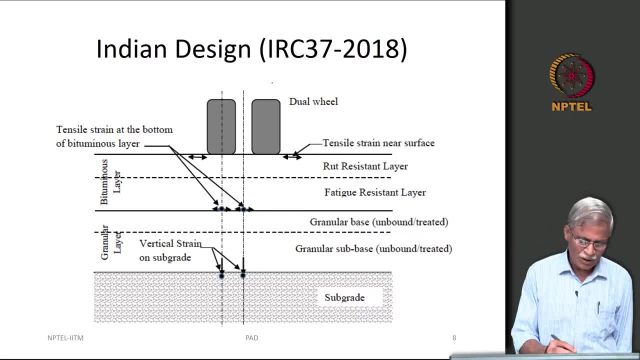 Now, there are many design aspects also that are introduced here, So let me just kind of give you a clue about what are these design aspects, These words that you see here. fatigue resistance layer. vertical strain on the sub-grade rut resistance layer. 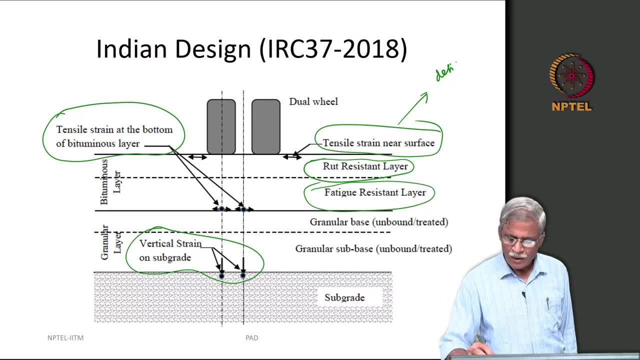 So all these things that are written in green color comes from the perspective of design. So first let us take a look at the cross-section. The cross-section is the same. You have a sub-grade. It could be an unbound or a treated ground. 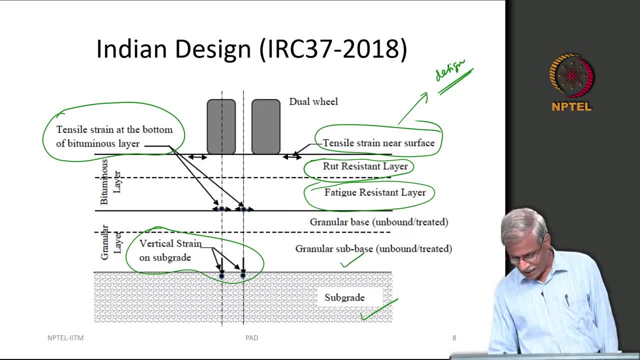 It could be an unbound or a treated ground, It could be a granular base. Now this sub-grade should be called as a what you can say as a compacted sub-grade. Then you have a base here and then there are two bituminous layers. 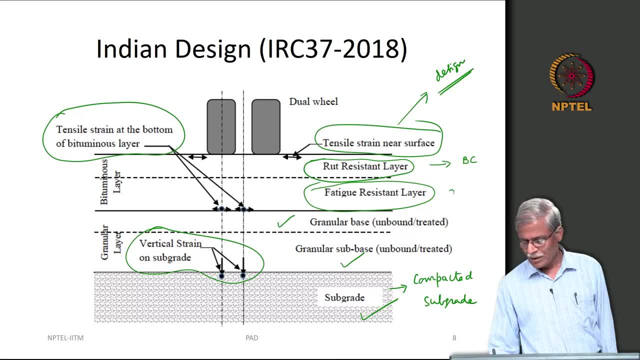 So what we call in India as bituminous concrete And this could be called as… Dense bituminous macadam. So there are going to be two grades here, depending on the binder content used and the gradation that is used here. Now let us look into the design aspect, what it says. 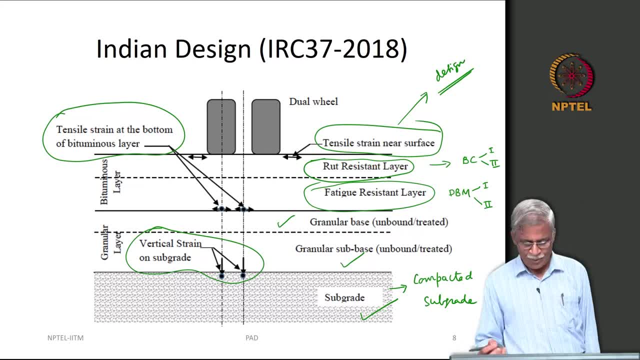 So, first and foremost thing is there is a common perception that this vertical strain that you see here, whatever that strain means, if is limited, there will not be any strain, There will not be any vertical strain, There will not be any vertical strain. 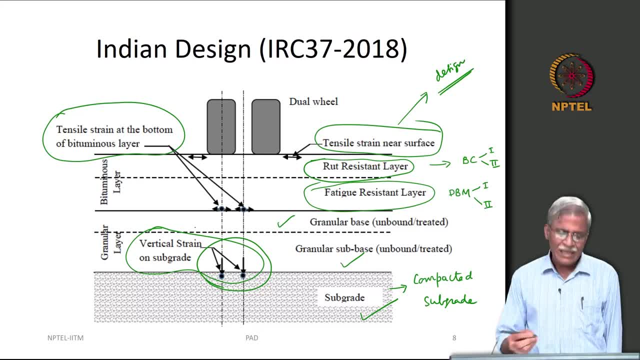 There will not be any what you can say failure related to rutting. We will see what are those rutting and fetting as we go along. Now, in the same way, if the strain at the bottom of the bituminous layer is limited, 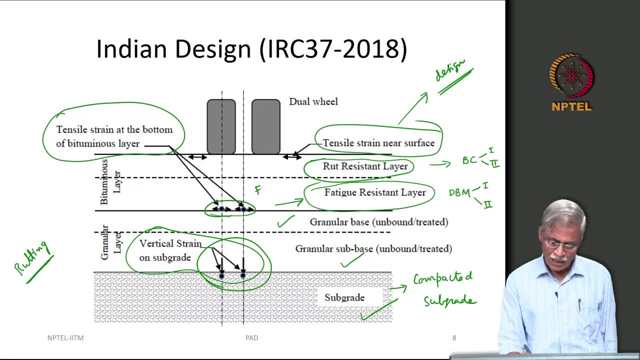 you can actually see that there could be less probability for the bituminous pavement to fail due to fetting Dense bituminous macadam, Dense bituminous macadam- And this also can happen at the top, So there is also tensile strain at the top, tensile strain at the bottom of the bituminous. 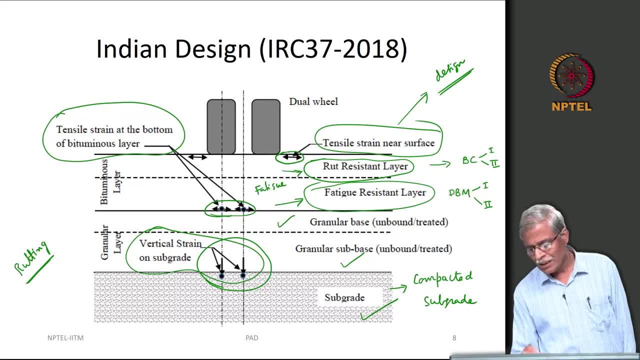 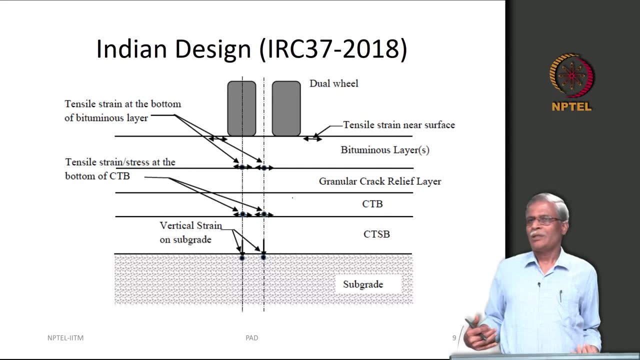 layer. So it is expected that you will construct these layers as rut resistance or fatigue resistance layers. So this is the general cross-section, with the design aspects also integrated part of it. There are many other cross-sections that are given in IRC 37.. 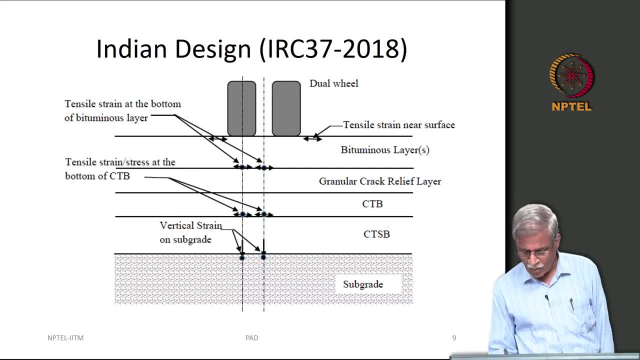 I do not advise to go and take a look at it, but I will just go talk about There is a cement treated sub-base. there is a cement treated base and because of this stiffness there is a necessity for something like a crack relief layer. and then the bituminous. 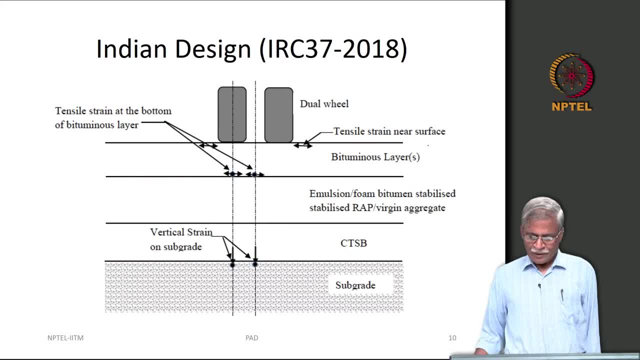 layer. Rest of the things remain the same. Then, in addition to that, there is also one more cross-section which we will be discussing as we go along. So it is about what is really called as cement treated sub-base, and this is the foam stabilized. 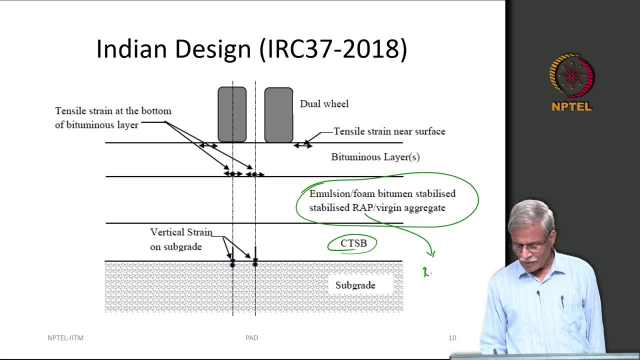 or so. this is your reclaimed. So if you constructed a bituminous pavement and if it requires rehabilitation, what you could do is to do what is really called as the full-dose. So this is the full-depth reclamation- and take all this material, add it with the new. 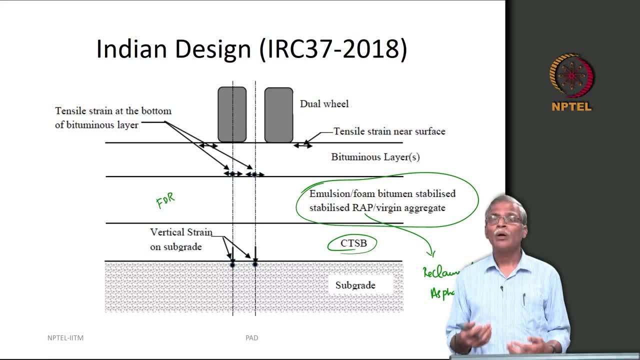 material, add a binder in the form of a foam or an emulsion and lay it here, and then on top of it you can have the regular bituminous layer. So there are many ways in which one can construct such cross-sections. 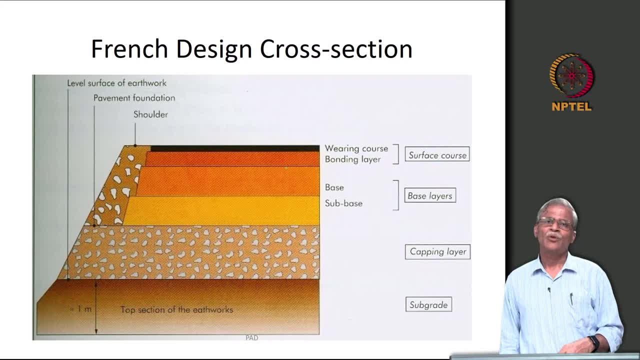 We will slightly go out and see what happens to the French cross-section. The French cross-sections are empirical works very well, So they do not give you much flexibility about what should be used. So there is a surface course, there is a base course and this is called as a capping layer. 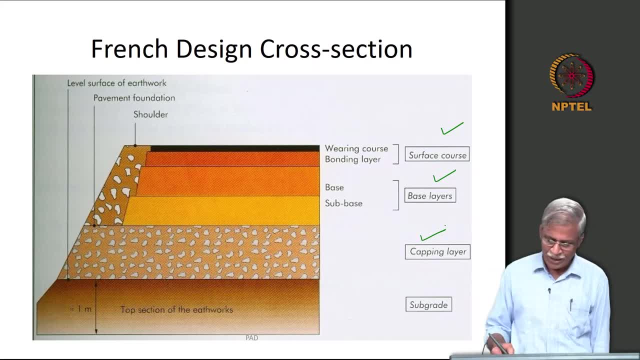 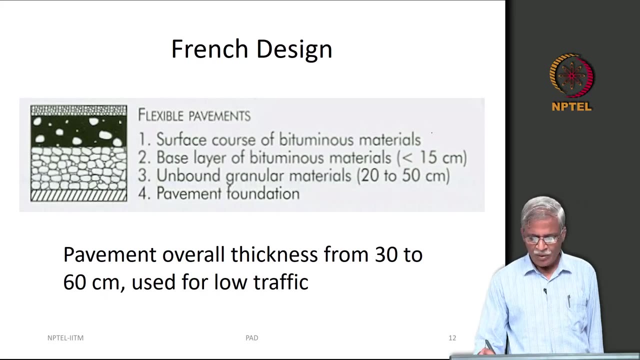 What is normally so. it could be a drainage layer, it could be anything, So this is called as a capping layer, and this capping layer is constructed on top of the sub-grade. and there are many design strategies that are followed. See, for instance, you can have surface course of bituminous material. 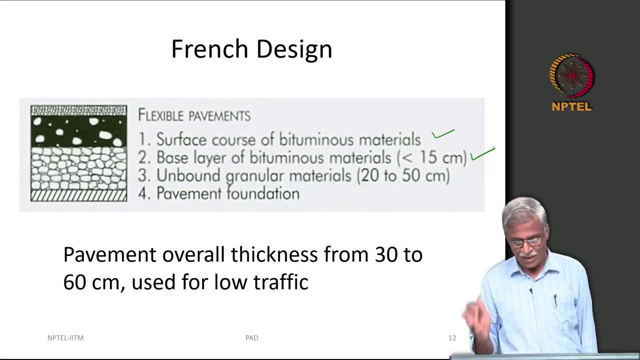 Base, Base layer of bituminous material less than 15 centimetres and, the most important thing, is unbound granular materials that can go as high as 50 centimetres, and this is what is really called as a pavement foundation. I have a reason for emphasizing all these things because, at the end of the course, what 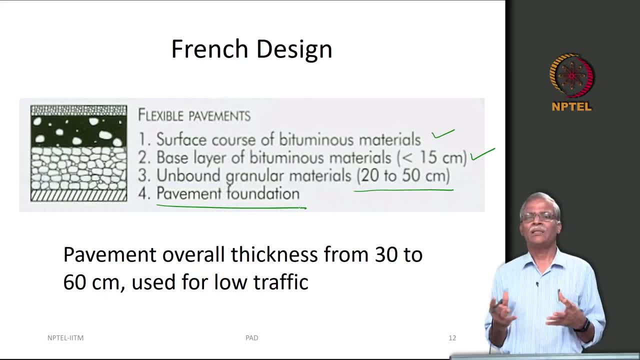 you are going to do is to take any of the existing IRC 37 cross-sections, use the distress functions, apply the load, compute the critical strain- Okay- And substitute this critical strains in this distress functions and see whether, whatever design, the equivalent standard axle load for which it has been designed, whether it. 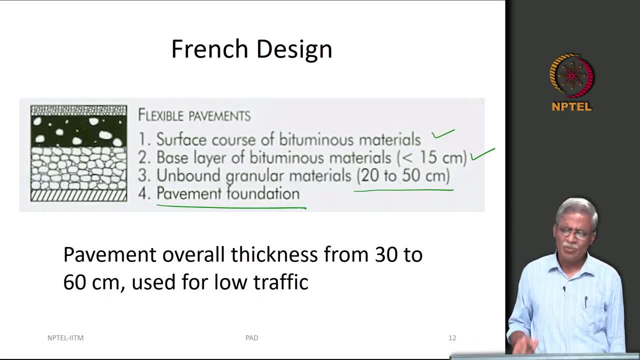 actually meets or not. you are going to check it and sometimes you will be surprised. So watch out for that right. So the same thickness could be for low traffic. I mean, the same cross-section design could be used for low traffic, medium traffic as well as for high traffic. as far as the French, 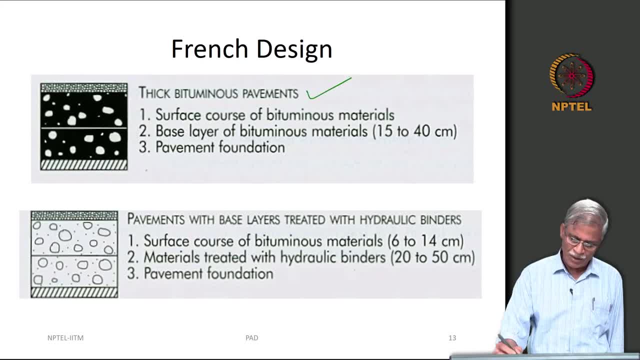 design is concerned, There is also what is really called as a thick bituminous pavement. Now, this thickness can go as high as 40 centimetres. So within the Indian context, you should be able to understand and appreciate it, because if you add up the total bituminous layers within the Indian context, we normally do. 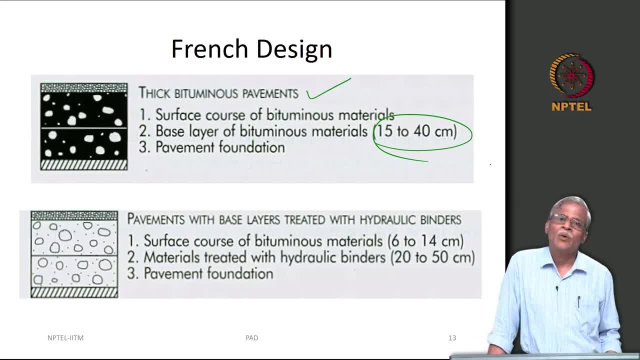 not exceed 15 or 16 centimetres, whereas these people want you to provide something like 40 centimetres, More than twice as much as normally. that is produced Okay, And there are also some cross-sections with hydraulic binders. 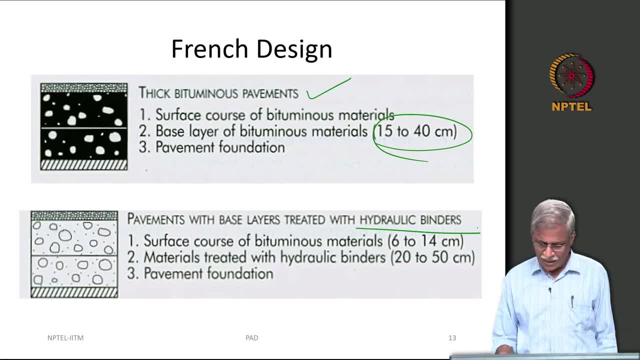 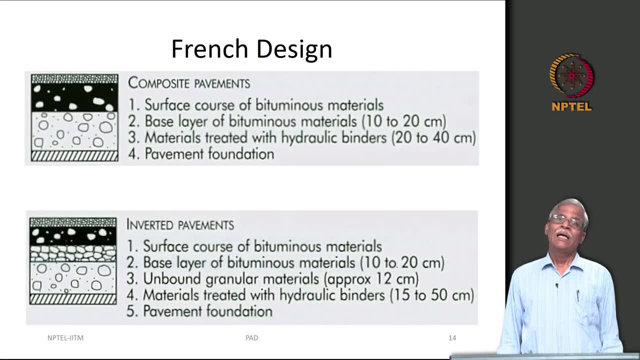 Hydraulic binders is nothing but using cement as a layer, So you can treat it, call it as a cement-treated sub-base or cement-treated base. In addition to that, the French people also have what is really called as a composite pavement, So you can have bituminous layer surface and base, and then you can have a 40-centimetre. 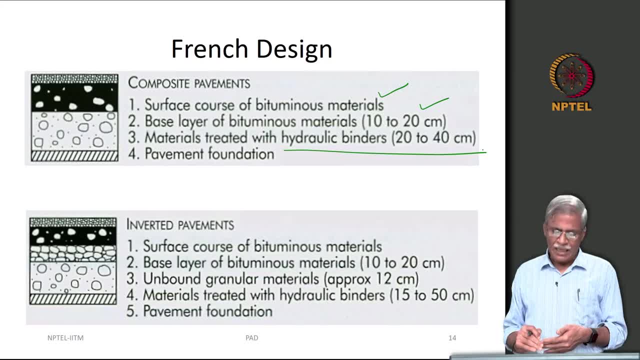 thick cement-treated base. Okay, And again you can have what is really called as the inverted pavement, in which you can have the material treated with hydraulic binder below, which has a lot more stiffness, and on top of it there is an unbound granular material. 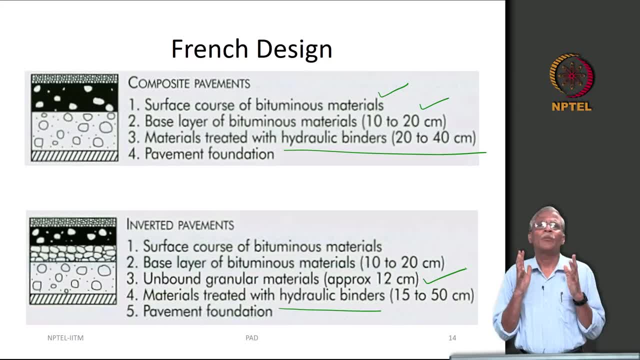 Now there are some issues related to computing the critical stresses and strain when you are using this kind of inverted pavements. Okay, It will become obvious as we go along, because the stress analysis procedure that you follow basically assumes that E1 is greater than or equal to E2, greater than or equal to E3. 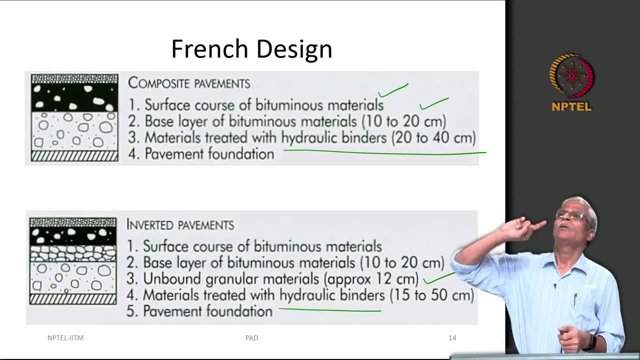 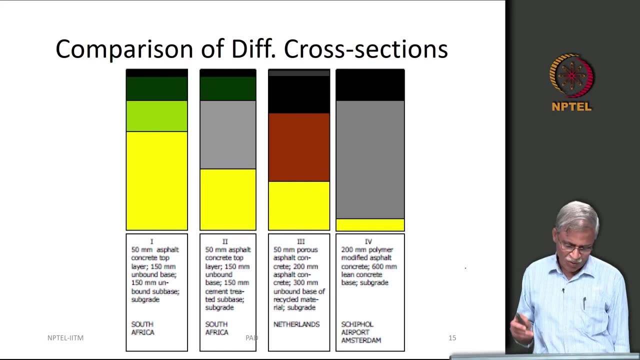 and so on and so forth. So sometimes, when you are going to have the modulus value of the bottom layer slightly more than what you see for the top layer, you might have some interesting scenarios we will see. Okay, So all these cross-sections, what you will see is: so there is a, you can see South African. 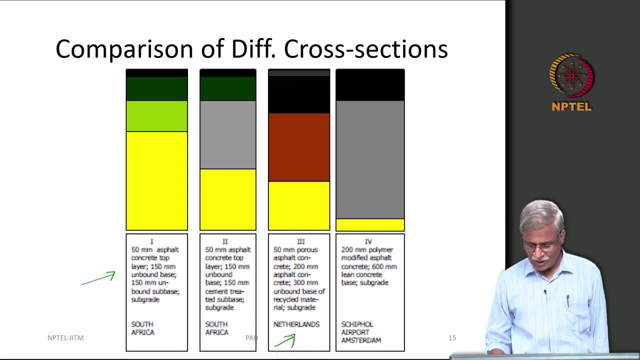 cross-section. then there is a cross-section from Netherlands, and this is a typical airport Amsterdam airport cross-section. So you see, there is a 200 mm polymer modified asphalt, 600 mm lean concrete base. So this is what is available as far as the Schiphol airport in Amsterdam: 200 mm, If you. 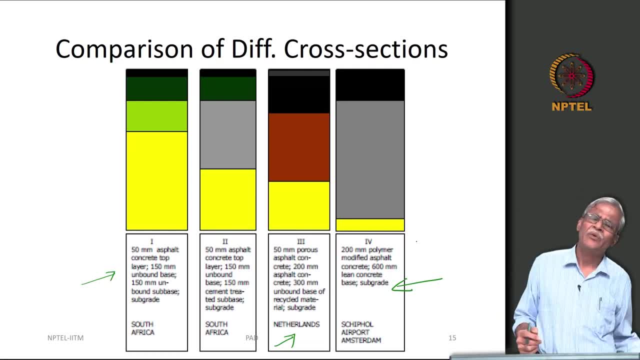 look into the Netherlands cross-section again. it depends on the country. when you are going to have lot of water, lot of rain, you are going to have some kind of porous structure that you construct at the surface wherein you allow the water to drain through and collect. 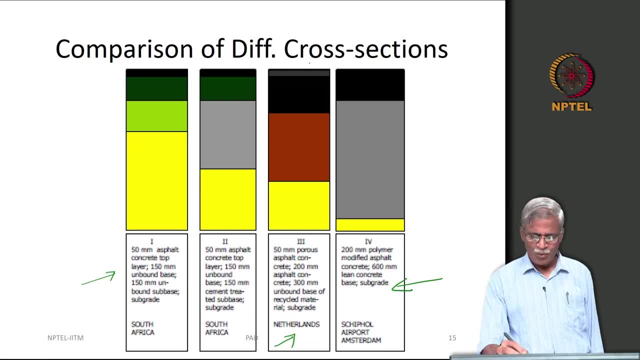 it through some of these drains. So you can have 50 mm porous asphalt concrete, 200 mm asphalt concrete and 300 mm of unbound base. But on the other hand, if you look at the South African cross-section, you can have 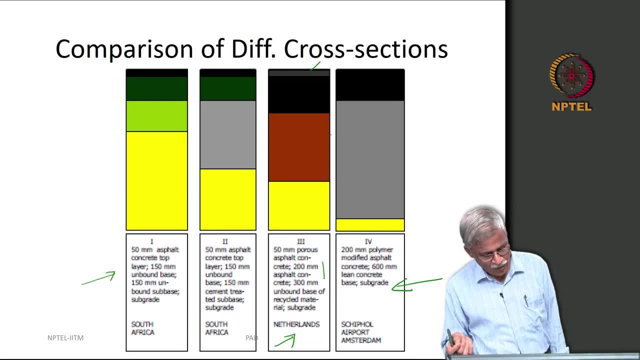 50 mm bituminous layer, 150 mm of unbound layer and 150 mm of cement treated base. So there are many combinations that are given, and now this is where I again want to emphasize to you about what is really called as proof checking, because most of these designs seems 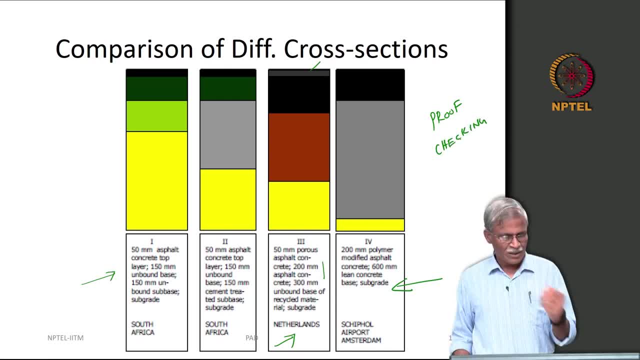 to have worked out already. You will see that you will be asking a question: so what is there to design? I have already worked out all the thicknesses. Now what you really need to find out is: what is the constituent here? What goes inside this material? number one: 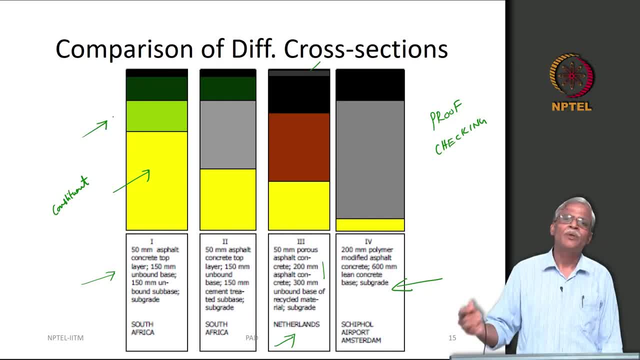 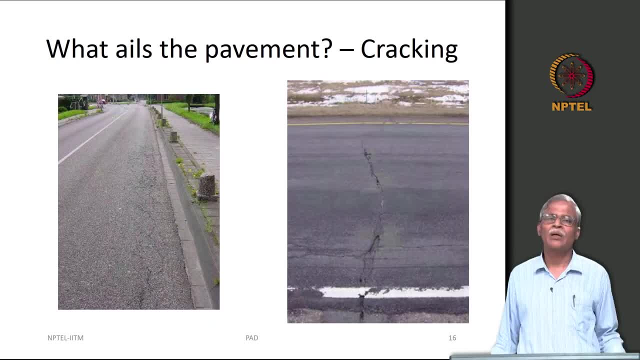 Number two is how long this pavement will withstand. So these are some of the issues that you will be able to answer. Now let us start talking about what really happens, and these are all nice pictures that you have seen. So there are going to be failures. 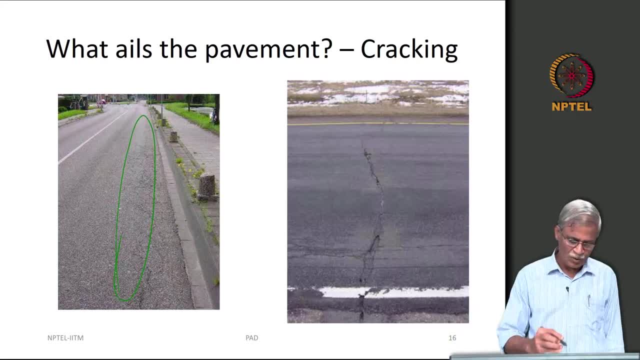 Now, These are the failures that are going to be a problem for you, because this is where you are going to be seeing here, So this is your traffic direction, So you are going to see what is really called on this right-hand side as low-temperature. 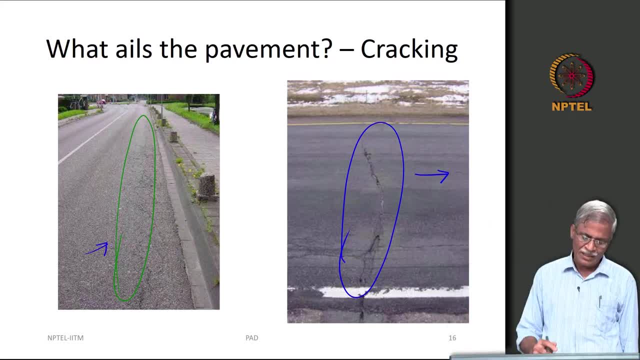 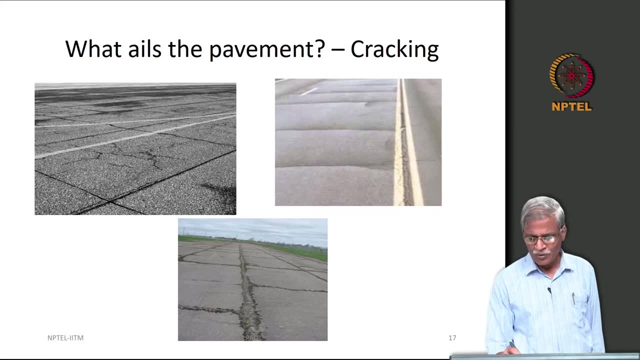 cracking and what you see here is the fatigue cracking. So this is the kind of cracking that can happen. There are many types of cracking. You can have most of this that form crack like a block. So this could be due to your low-temperature cracking. 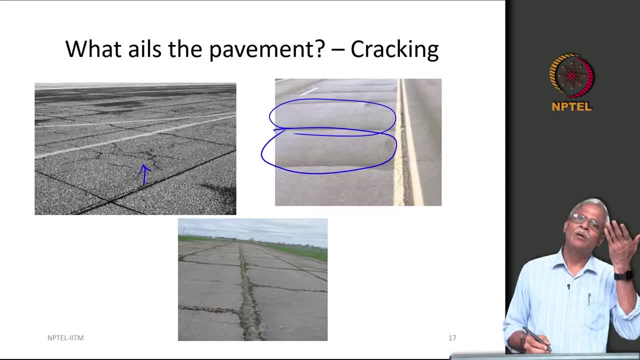 There could be some of these cracks that could emanate from the bottom and come to the surface, something called as a reflection cracking, And you can have many, many types of cracking. So what I would always call as two types: Load induced. 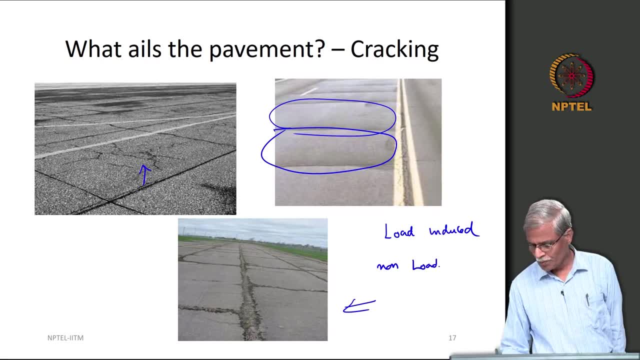 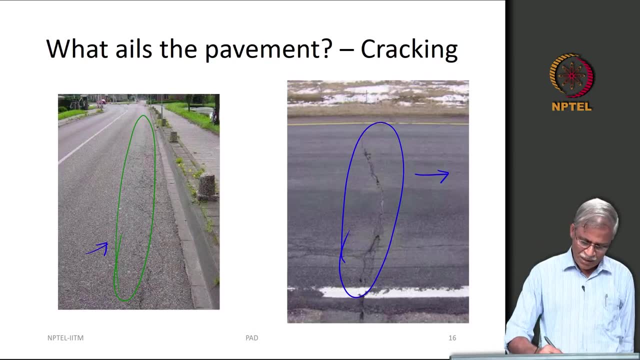 And Non-load induced. So that means if you are going to construct, let us say, a pavement, and you can think of it this way, So this could be, let us say, 2.5 meters. Now what will be around? sorry, 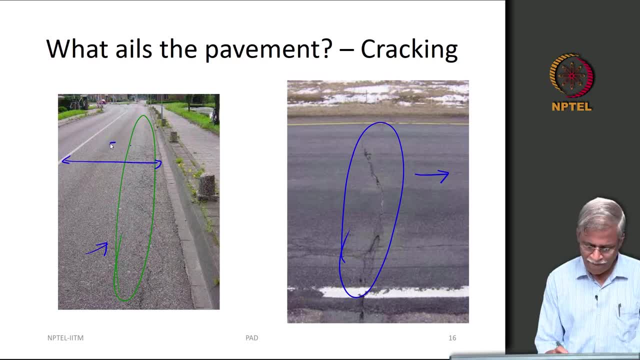 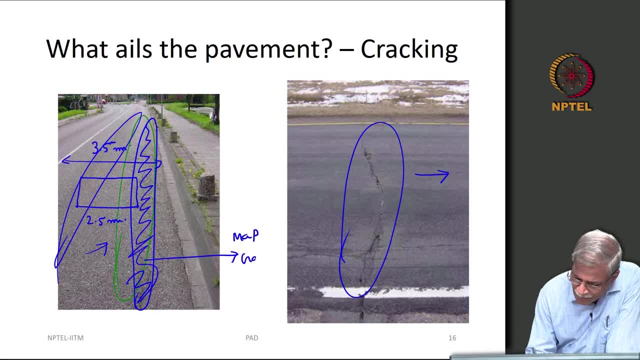 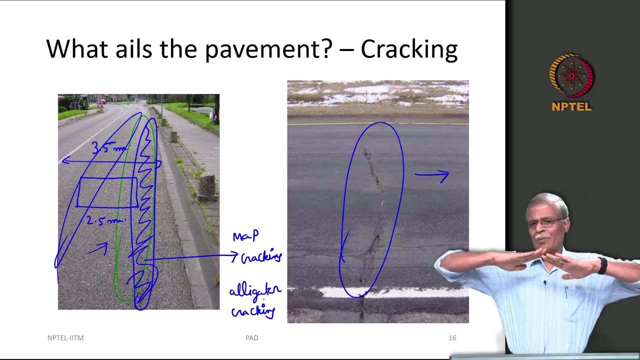 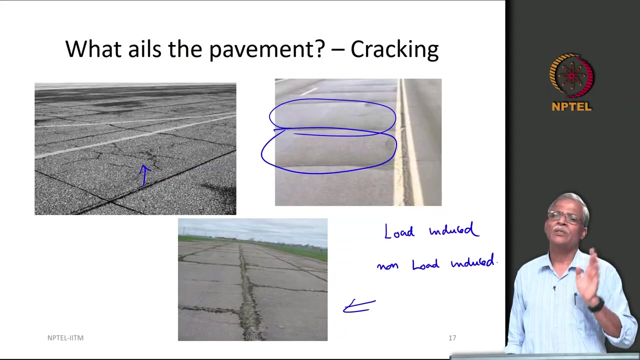 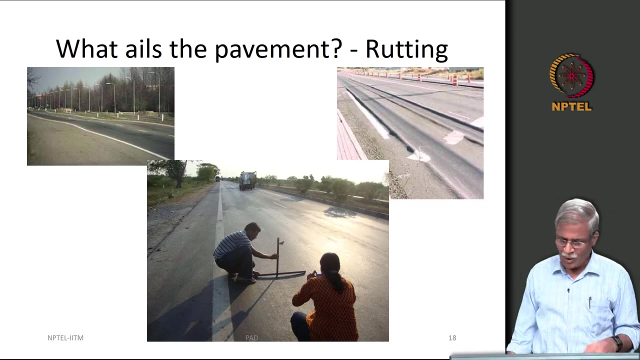 And you can actually see that this could be roughly 2.5 meters. So typically you know when you are driving the driver will position his vehicle. 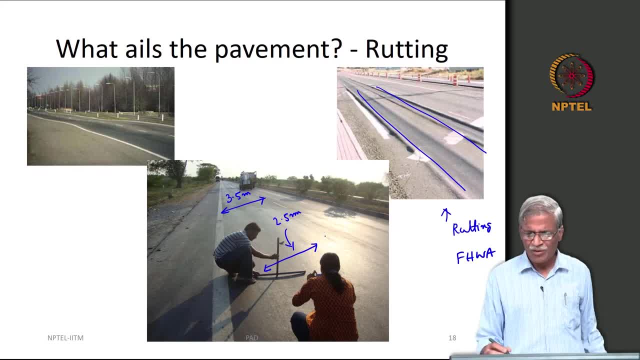 Let us say half a meter from this lane edge and another half a meter from the lane edge. This has something to do what is really called as the vehicle wander. So you are going to see that there is going to be considerable rutting here. 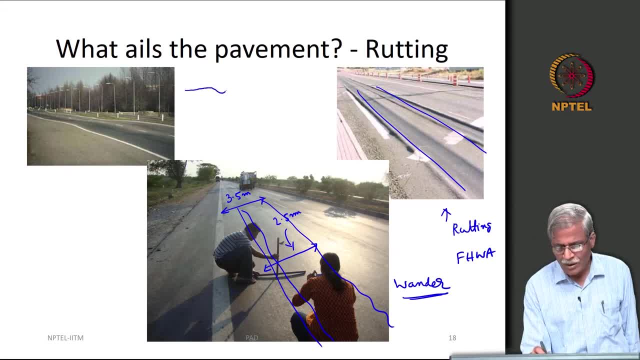 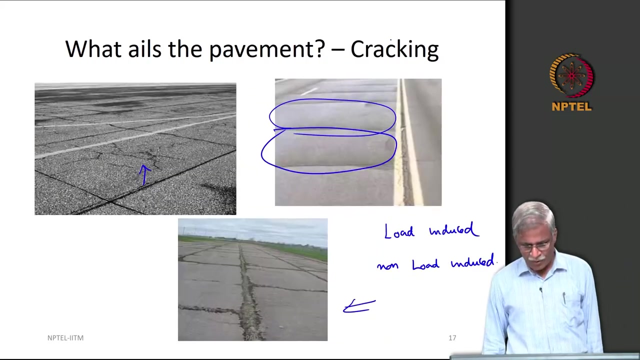 Now what will happen is, if you take a look at the cross section, you are going to see that there is a depression in the wheel path- wheel path depression. So this is what you are going to call it as rutting and, in fact, if you recollect the 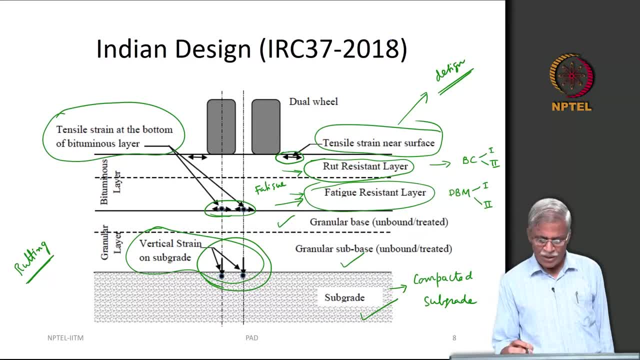 IRC 37 cross section. you will notice here that the topmost layer is designed to be a rut resistance layer. but they also tell you that if you limit the vertical strain on the subgrade to some specific value, we may not really have the expected rutting. 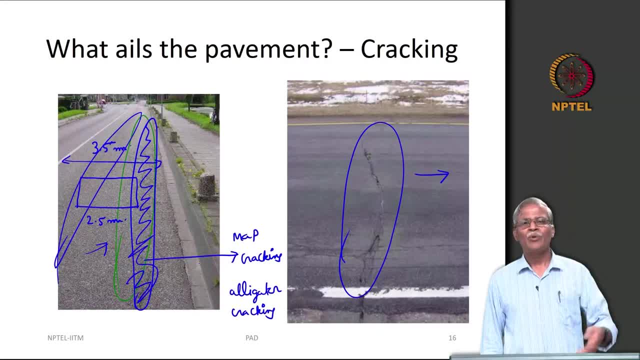 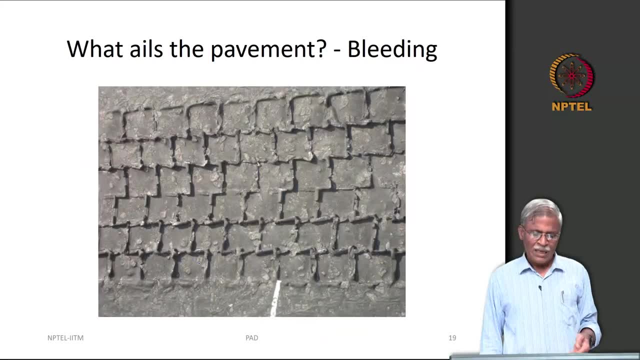 So that is a story that we will, slowly, we will be able to unravel as we go along, because I just wanted that The first lecture give you a flavor of what we are going to do here. Then you can have bleeding which is due to poor mix. design means using an inappropriate 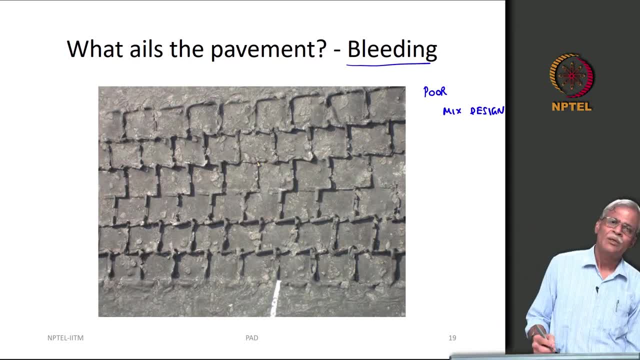 bitumen at a specific location, So you using a VG 30 bit, VG 10 bitumen where you should be using a VG 30 bitumen, or using a more binder content than what is needed, Or not providing the enough aggregate gradation fines and all those things. 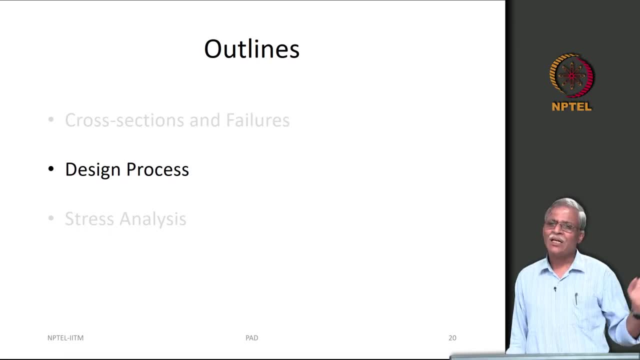 So this is more or less a general overview that I really wanted to talk about. So what did we talk about? We talked about the cross sections, We talked about the failures, and as far as the failures are concerned, let me list everything. 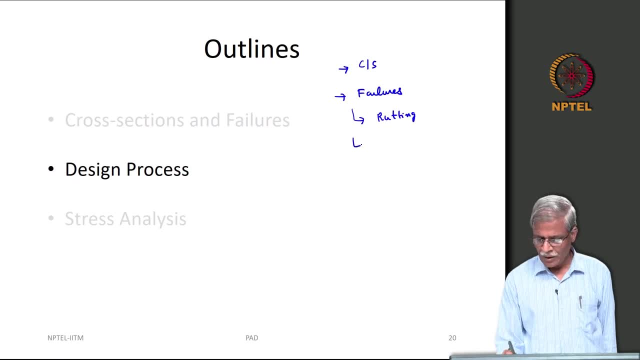 So you can have rutting, You can have fatigue damage, You can have low temperature cracking, You can have moisture induced damage. But normally when we talk about chirp, the failure in bituminous pavement, especially relating it to the cross section, we will 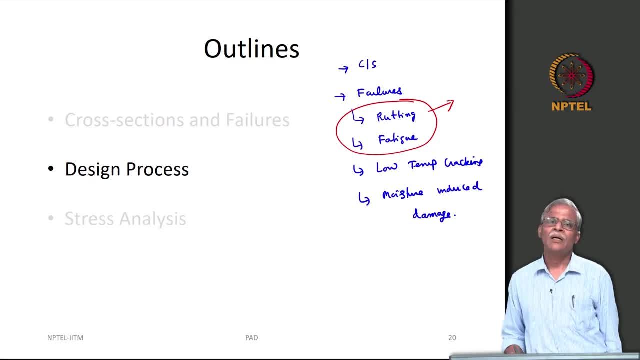 be focusing our attention on rutting and fatigue And in the IRC 37 cross section we also saw that there was a rut resistance layer. there was also a fatigue resistance layer and you also saw that the critical strains related to this rut resistance and fatigue resistance were measured for rutting at the bottom of. 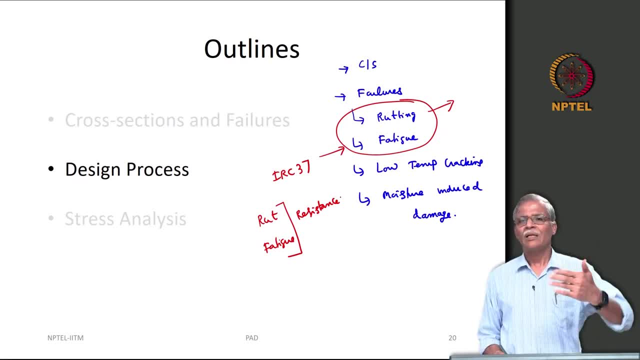 the pavement or on top of the subgrade and for fatigue, at the bottom of the bituminous layer. So these are some of the earlier assumptions that have been made. These assumptions need not have to be true And you will be exploring it as we go along. 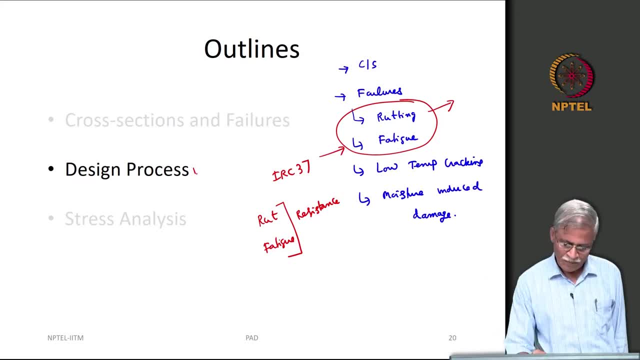 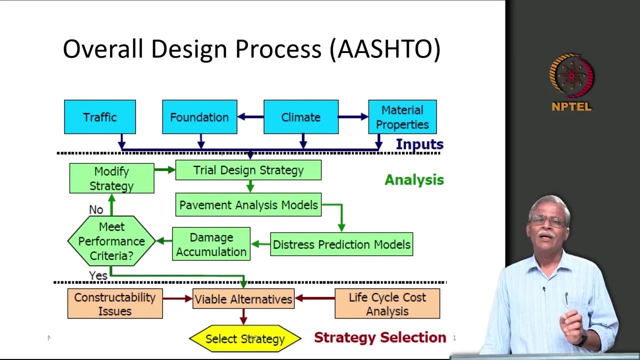 Now let us understand what is really called as the design process. Now this needs to be discussed in detail, and you will see that over the period of this course, 3 of my colleagues are going to cover different portion of it. Now let us define this separately. 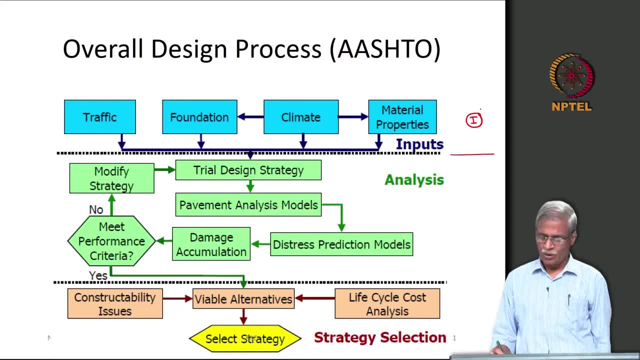 So this is the input, This is the flow rate that you are going to give, This is the analysis that you are going to do And this is, finally, the strategy selection. So what each of this basically means. So let us assume that you are going to construct a bituminous pavement. 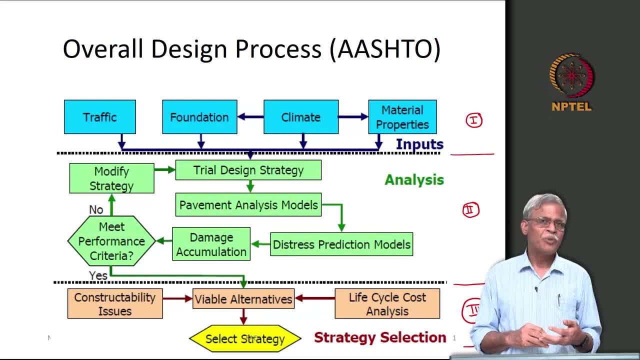 Now, this construction could be a brand new pavement, or it could be widening and strengthening an existing 2-lane road into a 4-lane road or a 6-lane road. Right, it could be anything. Now, first and foremost thing is: what is that you want to really ask? 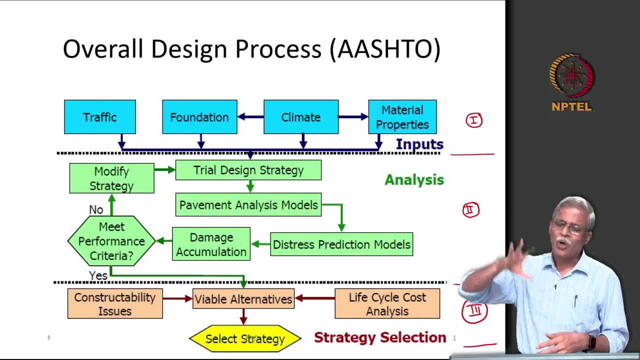 and please understand this design process, not only necessary to be followed for pavement engineering, but for any civil engineering structure for that matter. So here, the load that is coming here is your traffic, So that is the most important thing. So when we are talking about traffic, we are talking in terms of two things: What is really? 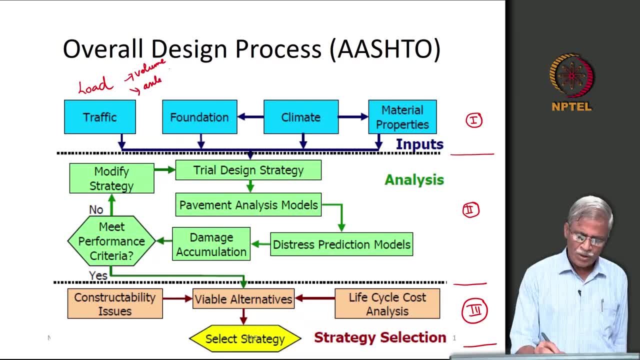 called as the volume count, What is called as the axle load. So when I say axle load, what are the different types of axle combinations that you are going to see and how, each of this truck having a different combination of axles, what is the total number that you 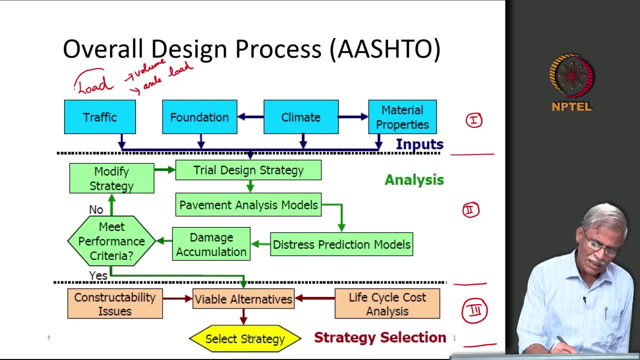 are going to talk about. Okay, So that comes under the load or traffic. The next thing is: where is the road going to be constructed? What is the load carrying capacity of the existing soil, So what we really call as the foundation? Now, this is where I want to keep making the distinction as we go along. 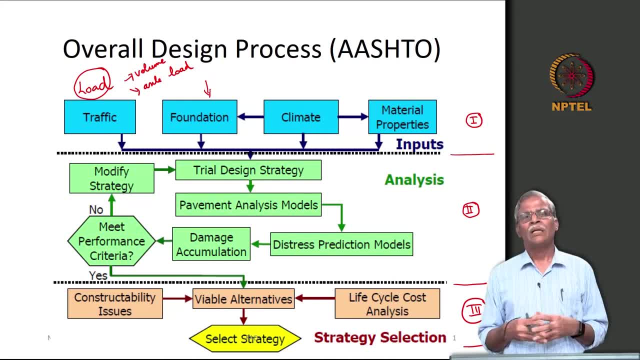 So when you are going to construct your bituminous pavement, depending on the country you live, you will want to find out the CBR value of the subgrade, The contents of the subgrade of the road where you are constructing it. you are going to find out the CBR value of 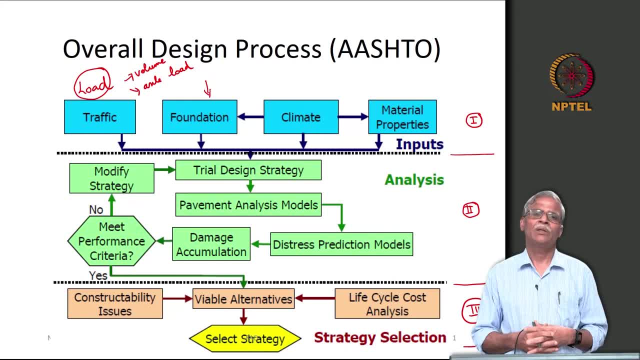 the subgrade, If it is going to be for bituminous pavement, if it is going to be for concrete pavement, they will tell you, go find out the modulus of subgrade reaction. The soil is the same. The road that you are going to construct has only some changes in. 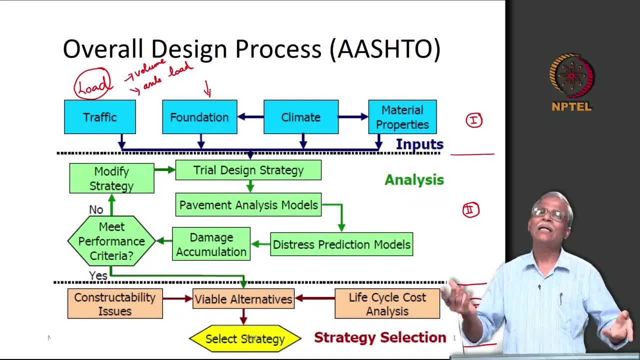 the constitution, the layers, type of materials that you use. But since the stress analysis procedure demands modulus of subgrade, I will say that it will be the same. You do not have to usher in the road as you would. I don't want to be the one to be worse than the other. 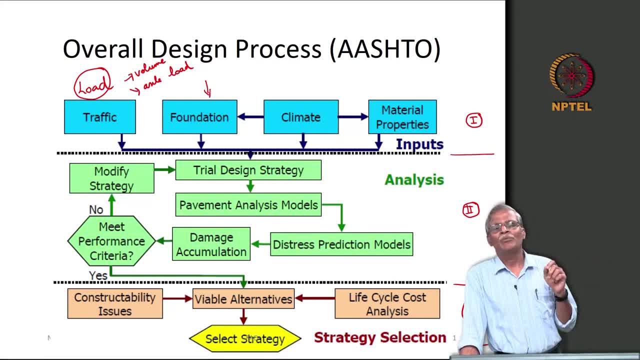 So in this case, that is what I have been talking about. So here, this is the level of soil mal depuis, of subgrade reaction for concrete. you will be measuring the same for the subgrade material, But for the same subgrade material if you are going to construct a bituminous pavement. 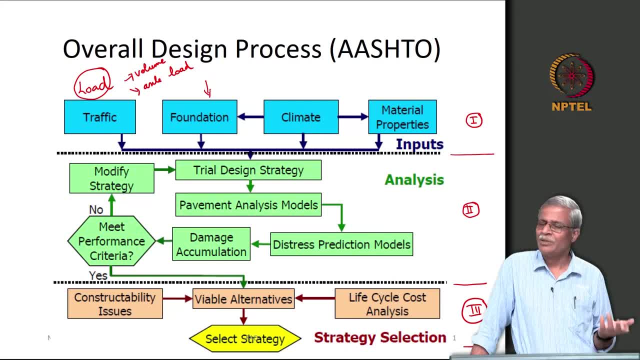 you are going to find out some CBR, some resilient modulus or something like that. So the most important thing is: what is the foundation? You can say the load carrying capacity, And this is where you will also be able to relate that what is called as a compacted subgrade. 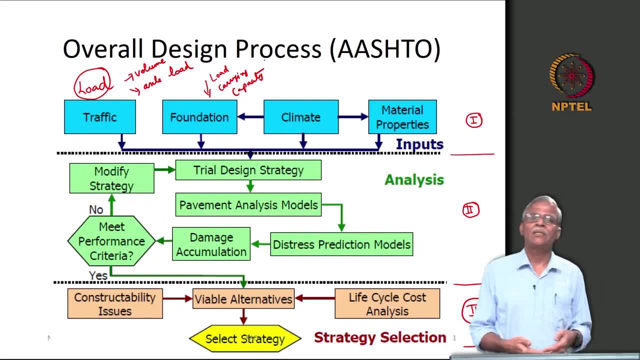 So many of the design charts that are given in IRC 37 talk about the thickness to be provided on top of a subgrade having 10 percent CBR. Now what will really happen if your actual CBR of the road is 3 percent? So that means you are going to constructed a compacted subgrade. 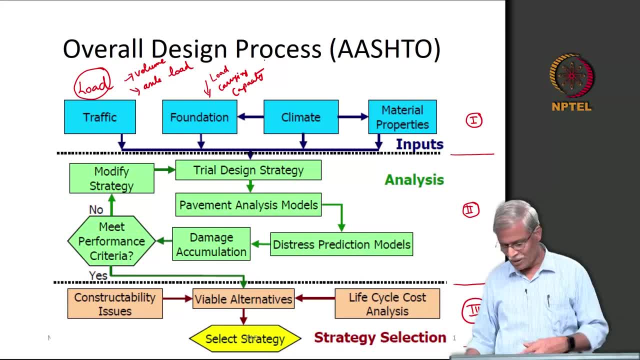 such that it will have a Subtitles by Prof K Ramesh, IIT Madras, around 10 percent or 15 percent CBR, Simple. The third and the most important thing is climate. Climate plays a critical role, more so in the within the context of India, because 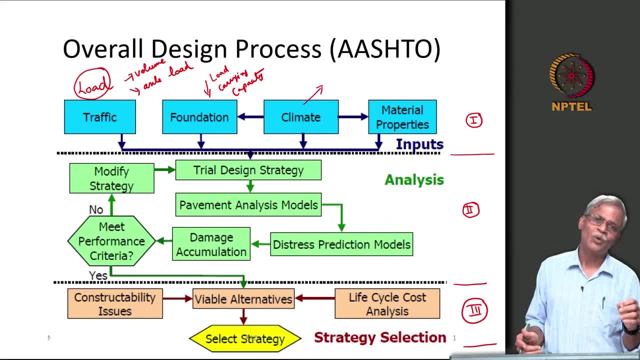 what will really happen in India is, whatever the cross section that you are going to use in the northern part of the India may not necessarily work out in the southern part of the India or the eastern or the western part of the India, because it has something to do with the maximum pavement temperature. minimum pavement temperature- presence of 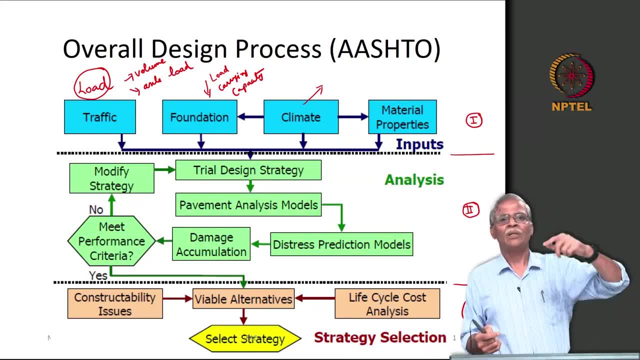 the water table and so on, And this depending on the temperature. the material properties, especially the bituminous properties, also will change, which means the load carrying capacity will change, which means the damage accumulation also will be at a different rate at a different month time period in a year. Climate plays a critical role. 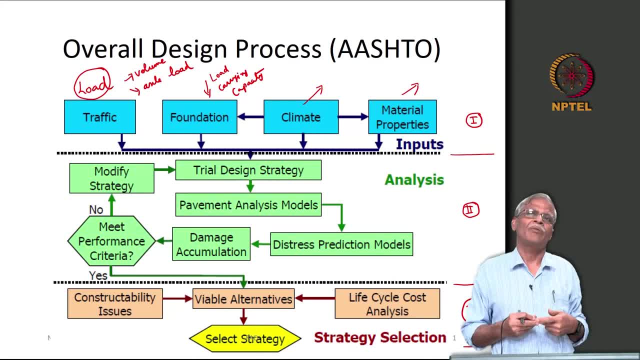 And then the material properties. are you going to use unmodified bitumen, modified bitumen? are you going to use stabilized base? stabilized sub base crack relief layer? what are its properties and everything? So this are the various inputs that you need to have. So that means before: 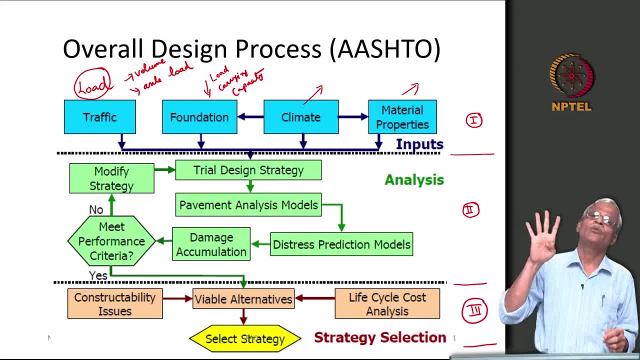 you start designing your pavement, you need to have these four things in your hand: The traffic, the foundation, the climate and the material properties. So, after having found out all these things, we go to the next step, which is the analysis. And now this is what I said: There is a trial design strategy that you need. What is the 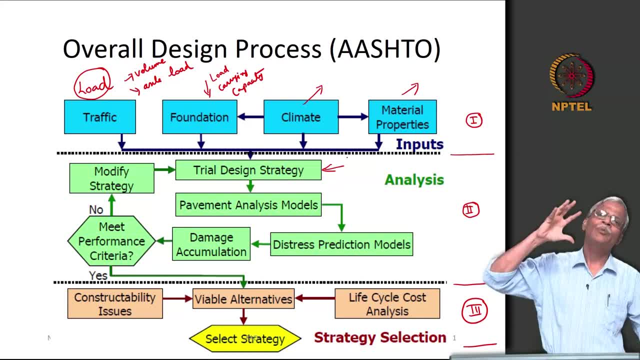 trial design. So that means we already have a clear cut idea of what should be the thickness of each of this layer. So it could be a bituminous concrete layer, 40 mm. Why 40 mm? Because your nominal maximum aggregate size may be 13.2 and typically 3 times the nominal maximum aggregate size is. 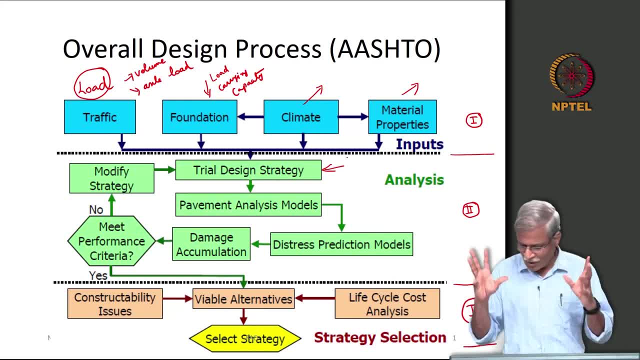 what you are going to use for your layer thickness. So 40 mm more or less comes there. So you take the trial design and then there is something called as the pavement analysis model. What exactly are this analysis model? So that means, given any pavement cross-section, how do you compute the critical stresses and 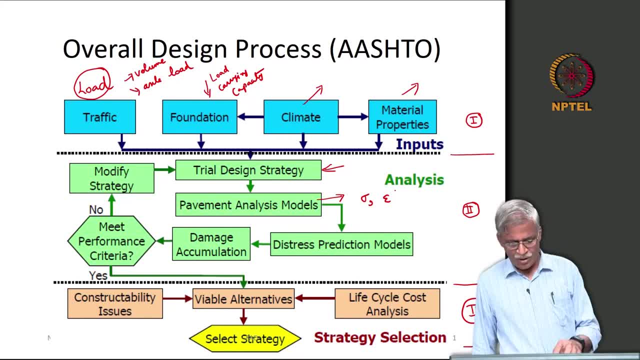 strain at a different spatial locations. So this is what is really called as pavement analysis models. Then after that, what do you do is you come to the distress prediction models. So we will be explaining as we go along. So that means for this pavement cross-section: 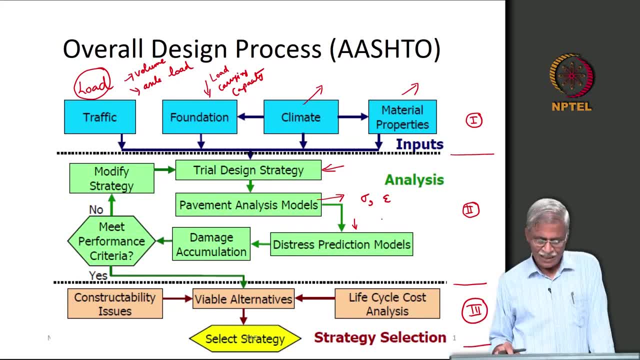 That you have taken as a trial, with the material properties that are given as input and using a computational mechanics procedure that you are going to follow, What will be the critical stresses and strains and how these critical stresses and strains can be related to the expected life of the pavement in terms of rutting, in terms of. 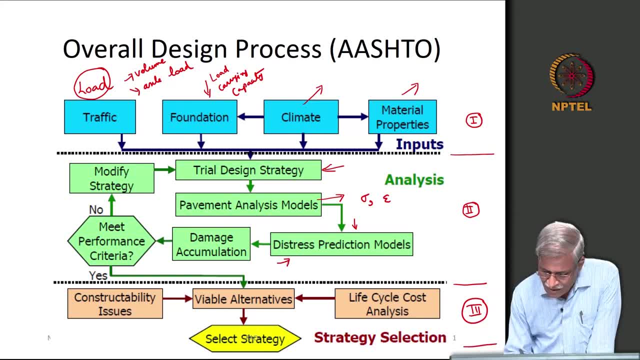 pavement. So this comes under the distress prediction model. And then, finally, what we do is we do the damage accumulation and when you do the damage accumulation, you basically are checking against your estimates that you made in air traffic with the trial design that you have taken. 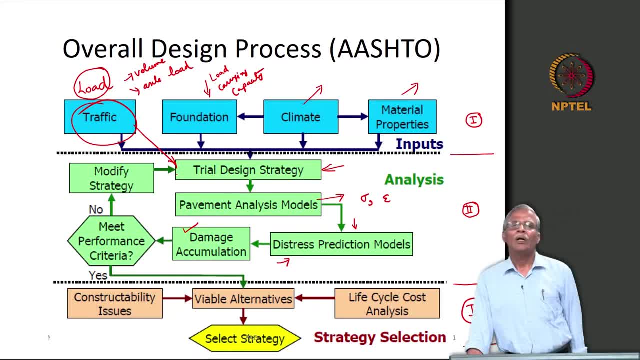 So let us assume I do not want to use the load equivalency factor here because it has not yet been introduced. Let us assume that I am designing a road for 1000 trucks, Just giving a simple example. So this is the traffic part that comes in, and I take a trial design strategy and after: 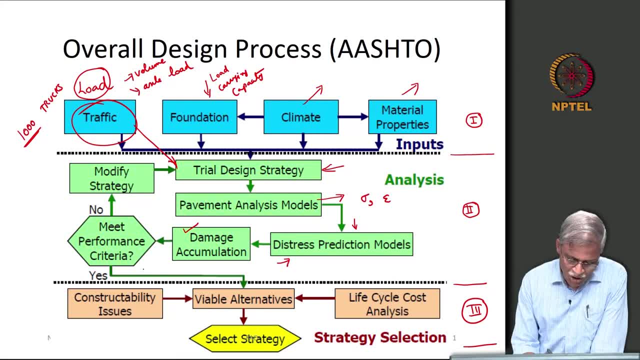 doing all the calculations, I realize that, oh, this can withstand 1200 trucks. So what you really do is you immediately say yes, But let us say You find out that, oh, this cross section can actually take only 900 trucks. Then what you do is you modify the strategy. 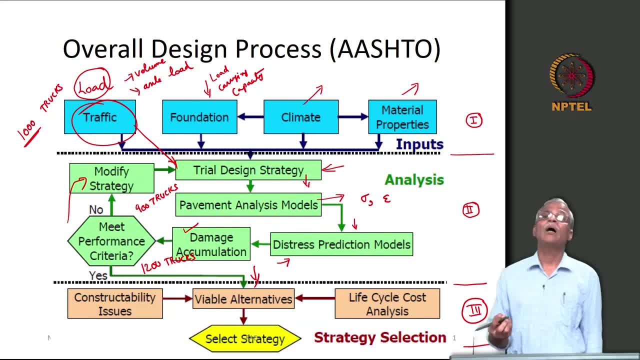 So that means you probably increase the thickness or you increase the modulus value of the constituent layer by using, let us say, polymer modified bitumen or anything like that, And then you come to the next stage. So this is a iterative process, as can be seen.